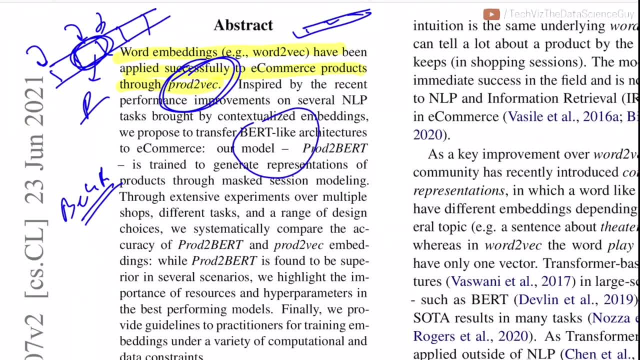 learning these representations, What is the trade-off in terms of time, How much data would you need, And what are some other practical considerations that you should keep in mind while choosing either of these methods? So yeah, that's what they have also written. 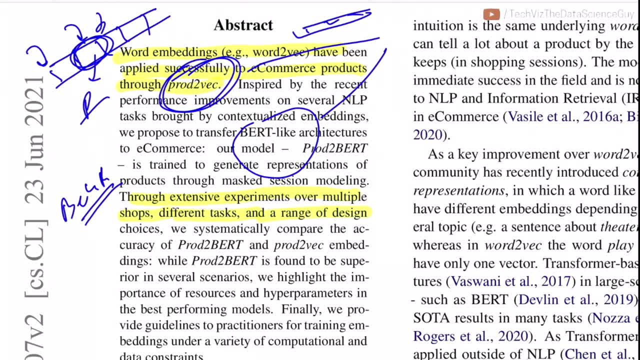 Through extensive experiments over multiple shops, different tasks and range of design choices, we systematically compare accuracy of prod-to-BERT and prod-to-vec embeddings. So yeah, that's the main idea of the paper. So let's move forward and see the rest of the details. 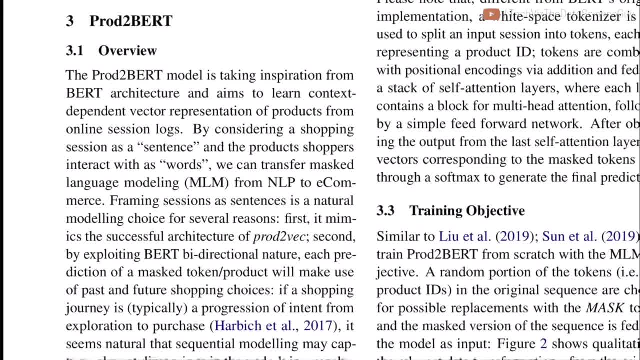 So for getting the BERT-based representation for each of the products, they train their model and name their work as prod-to-BERT, And the training is done in a typical fashion to how the BERT works, but just only the MLM part, which is masked language modeling. 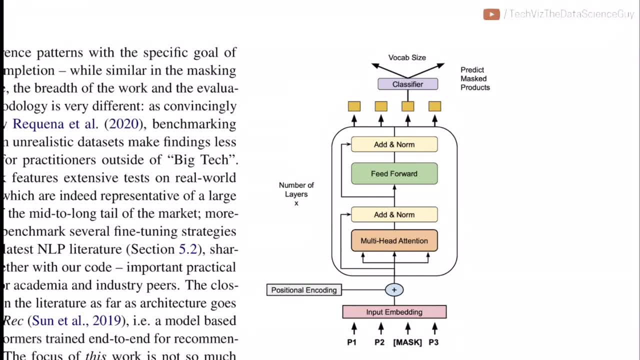 So, if you see this figure, the idea of MLM is to take a sequence of tokens- P1 to P3, for example, where some percentage of the intermediate tokens would be replaced with a masked token which will then be augmented by its positional embedding pass through. 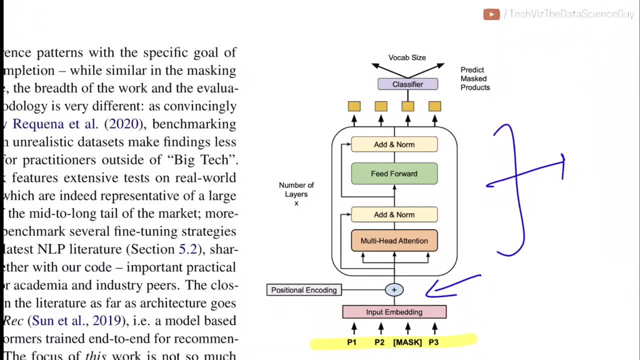 certain number of transformer layers, which are composed of multi-head retention and feedforward neural network, And at the output end you will have one representation per input where, at any given time, you will be predicting what is that word that can be placed against. 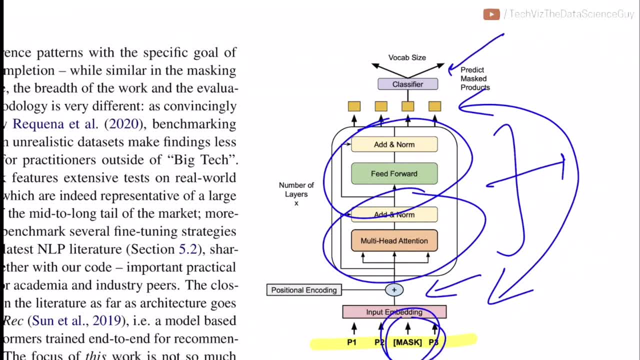 this masked token. For that you add a classifier, do a softmax, you get a probability distribution across the entire vocabulary and you choose the word that has the highest probability. So this is what we call a mass token. Now let's talk about MLM masked language modeling, Although the original BERT was also 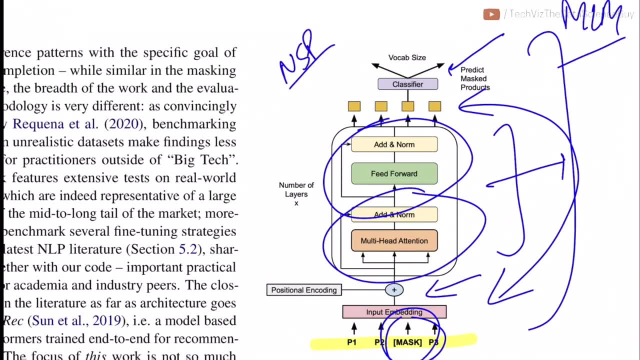 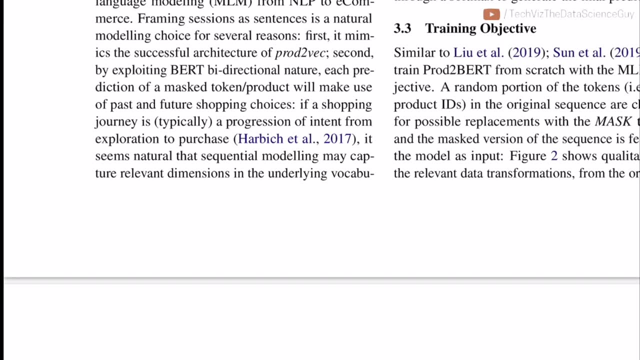 trained with another objective, which was NSP, which stands for next sentence prediction. But again for this use case, where we want to get the representation of every product given the search sequence, MLM was enough. So what they do is every session is now composed of a product that the user searches. So let's 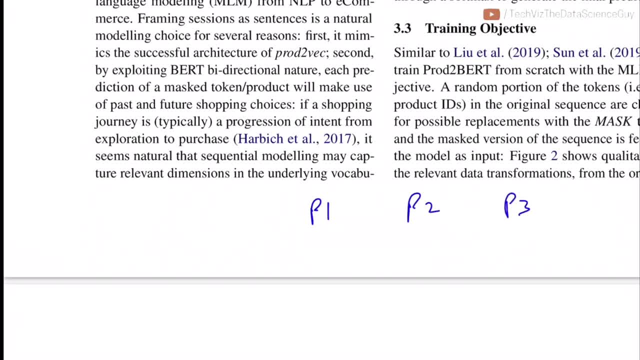 say, if I search for product number P1,, P2,, P3, and then P4.. This is one of the session If I log into my Amazon account, or any of that account, and these are the products that I searched through. So this is my search history for. 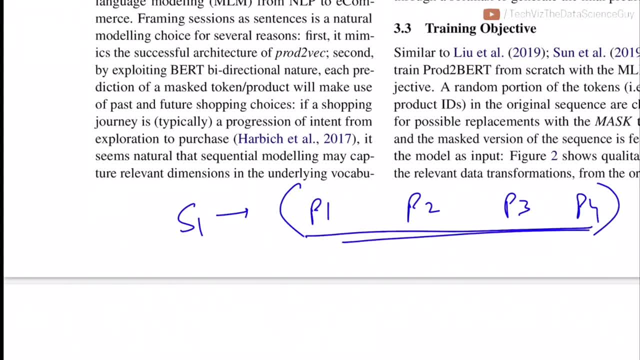 that session. So they treat every session as a sentence and each of these units, which are these products, as words in that sentence. And now the idea is same. You pass them through, BERT, and the output end. if, let's say this was masked, you try to predict what this word. 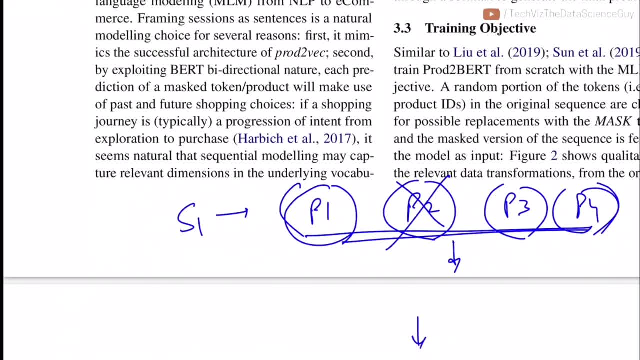 or the product was, And you keep iterating this for n number of sentences and also through duplicate instances of the same utterance. So that way you also capture the sentence level diversity in terms of the masked token. So if you see this figure again, let's say the first thing that you search for is the. 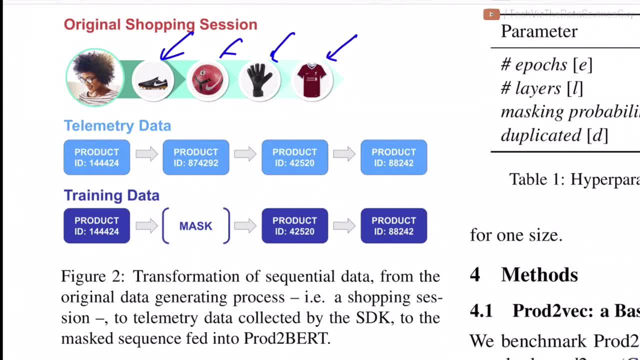 boots, then football, then gloves and then jersey. So this is what they call as telemetry data. These are the products that you had gone through. Now for transforming this sequence into the training data: you just mask some random 15 to 10% of the words and replace. 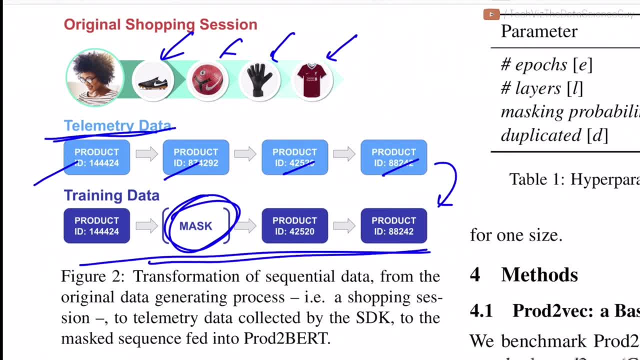 them with the masked token. This is what the sequence now you have, And typically you will find these sequences to be evolving over the intents, where the initial ones would be with the intent of exploration, And as you proceed towards the end, the chances are high that the intent has now changed to 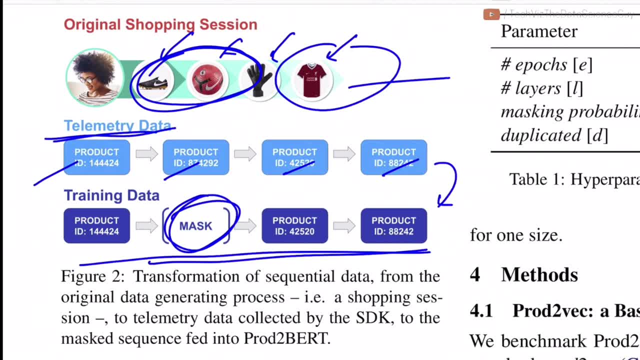 purchasing that product. So that way the sequentiality is still maintained, just like what happens in a sentence: flow, Cool. And once you have many of these training instances, you train your BERT model with the MLM objective which we had discussed earlier. 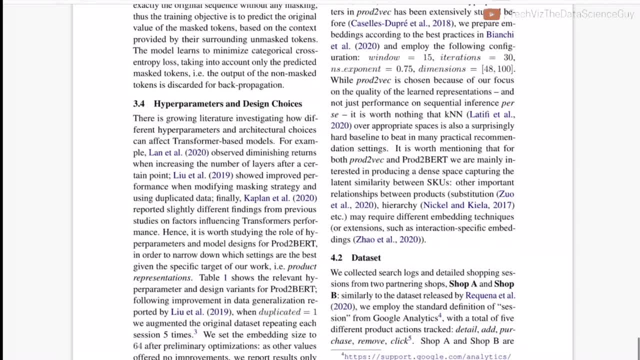 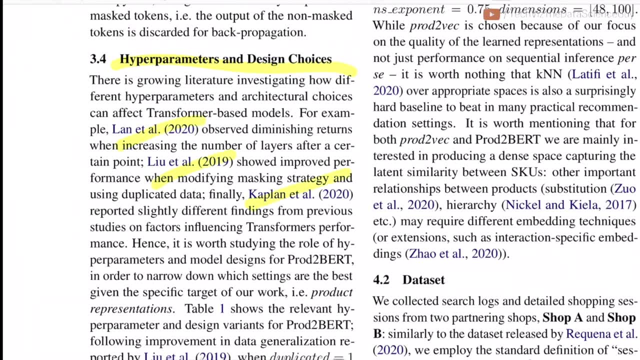 Okay, So now the authors talk about the hyperparameter and design choices. So under this section they discuss many previous existing literatures around how the number of layers affect the accuracy after a certain point And also, for example, let's say, whether the use of 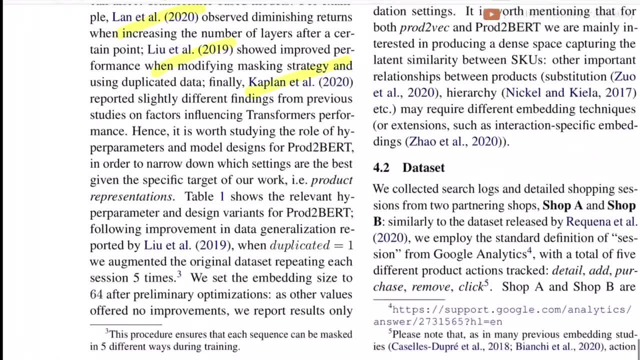 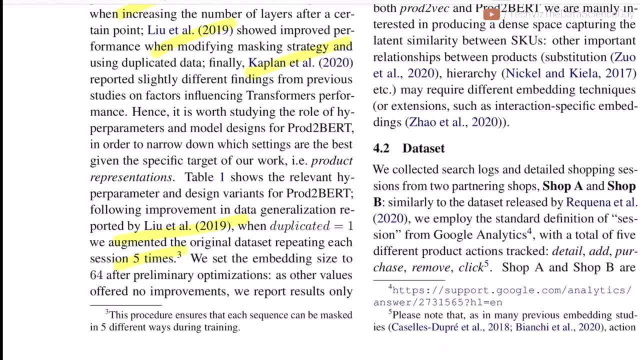 duplicate data helps in better generalization or not. So, as per Liu et al in 2019, they found that if you augment the data to a certain number of time, which is five in this case, the first thing which is obvious is that it gives you more data. So let's say you want. 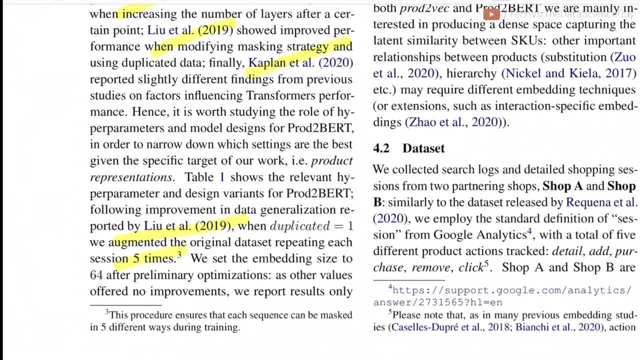 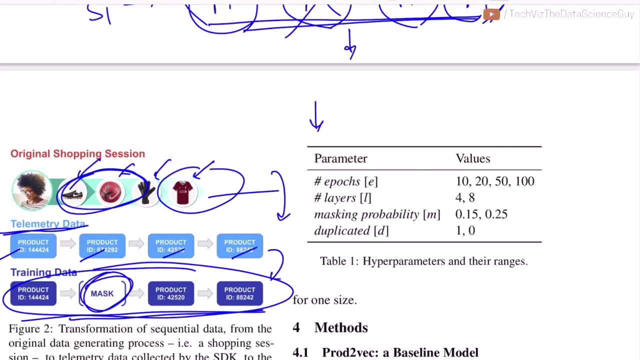 to use duplicate data, And with that it also allows you to kind of mask different segments of the same sentence during the pre-training phase. So authors in this paper also try that, And apart from this they also tune on other parameters such as epoch layers masking. 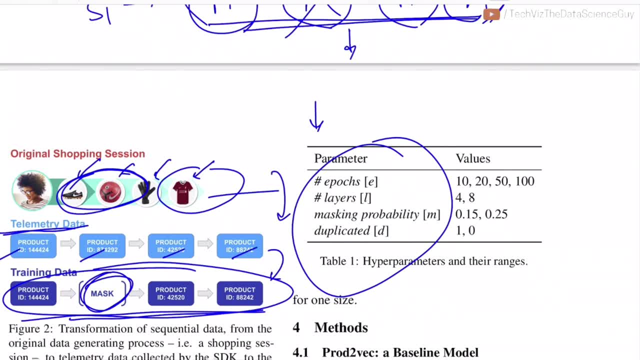 probability, as in how much percentage of a sentence would you put as a mask token and do the prediction for that. And then the duplicate, which is a Boolean value, whether they should be duplicated or not. So they use prod2vec as their baseline method. So prod2vec as 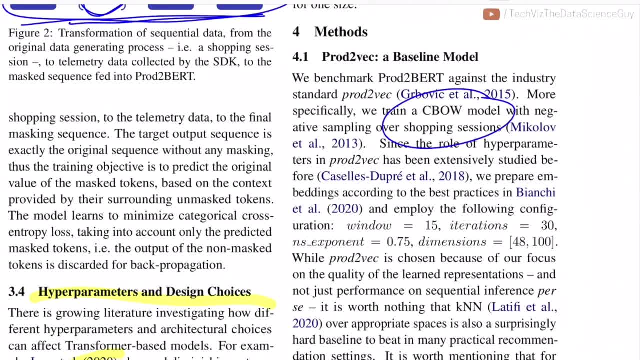 I had already discussed, is a very common method of duplicating. So what they do is they use prod2vec as their baseline method. So prod2vec, as I had already discussed, is a strain with the continuous bag of words: architecture, with negative sampling for all the shopping. 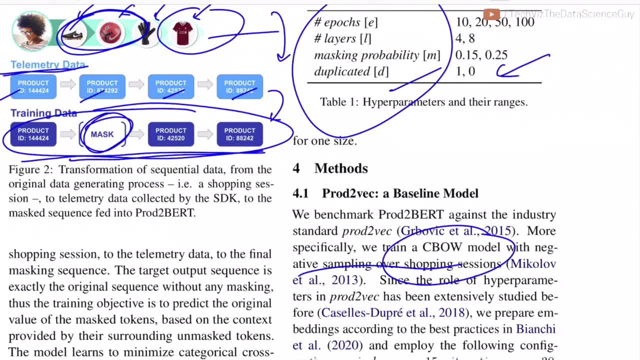 sessions, So at very high level. the way SIBO works is, let's say, if you have a sentence S that has these many number of words- one, two, three, four, five words- And let's say you want to get a representation for this. So we have a window length of two, which is 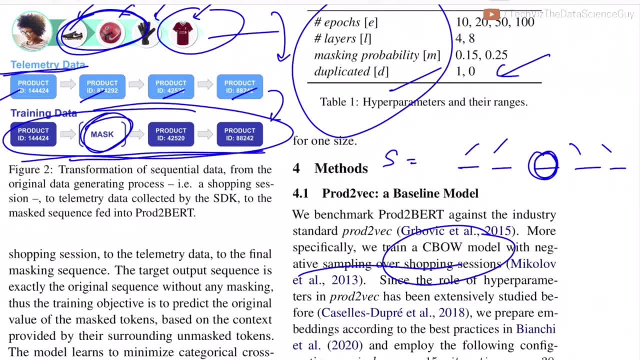 we will consider two words to its left, two words to its right, And at the output we'll utilize all these four words and make the prediction for the center word. So here you will have the softmax Over the entire vocabulary and based on how much you are close to the actual word, you'll 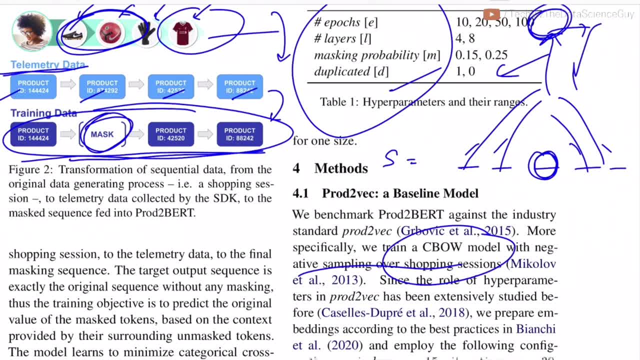 back, propagate and adjust the weights. So yeah, this is how SIBO would work, And negative sampling allows you to kind of put this target word in the context where it's not likely to occur, Cool. So, talking about the data set, author works with two data set from shop. 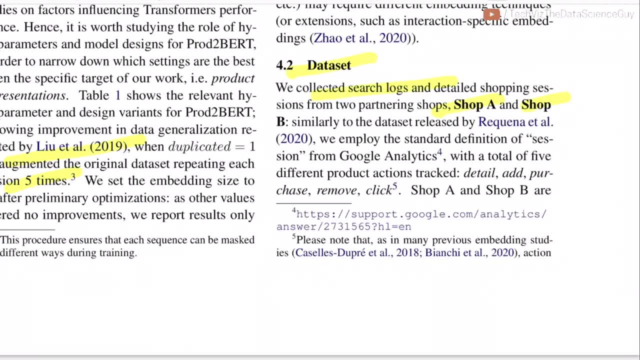 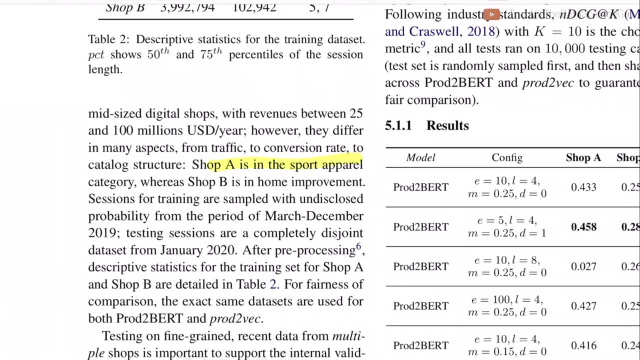 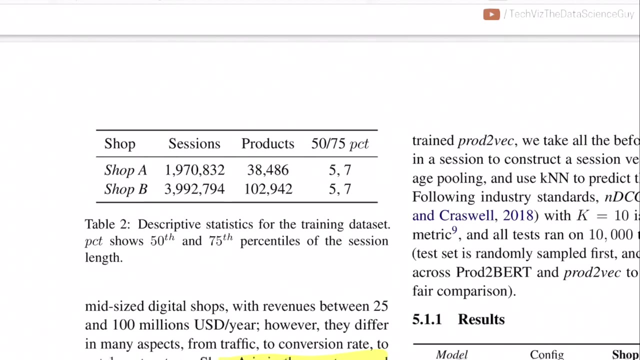 A and shop B, wherein they collect the search logs for each of these shops. that has around five product actions, And these are the four of the statistics that are listed over there. So, apart from this, they also impose a pre-processing step where they filter out any session that's less than 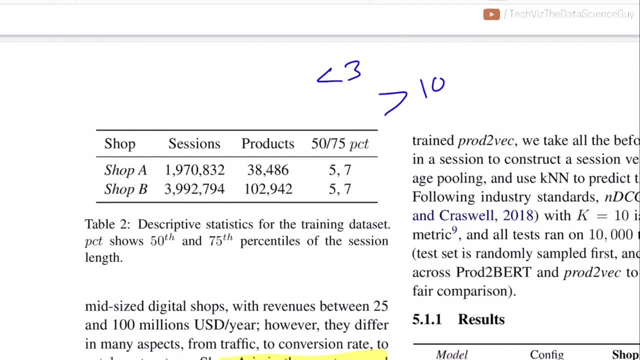 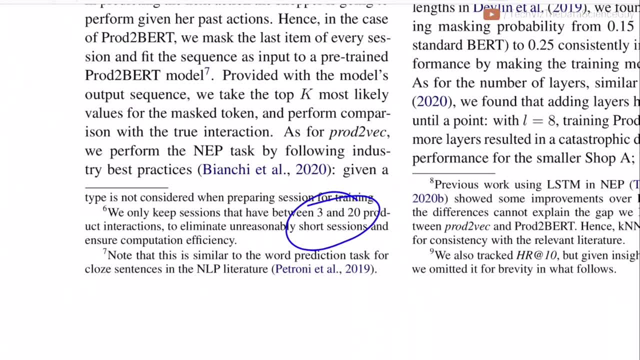 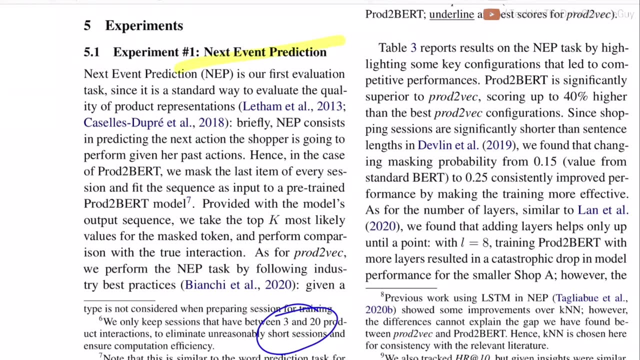 So, yeah, greater than 20 interactions. So if the sequence length of interaction is less than three, or if it's greater than 20, they eliminate such sessions. So that's about the dataset that they use. Then, talking about the experiments, one of which what they do is next event prediction. 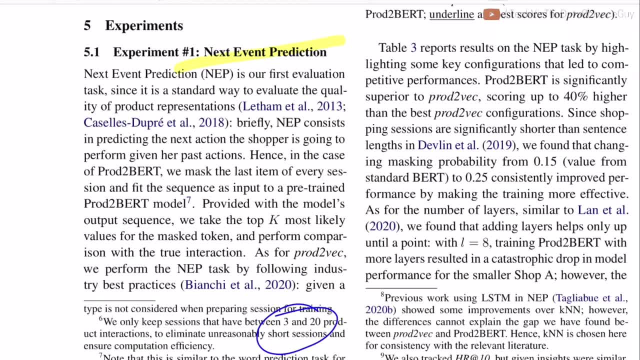 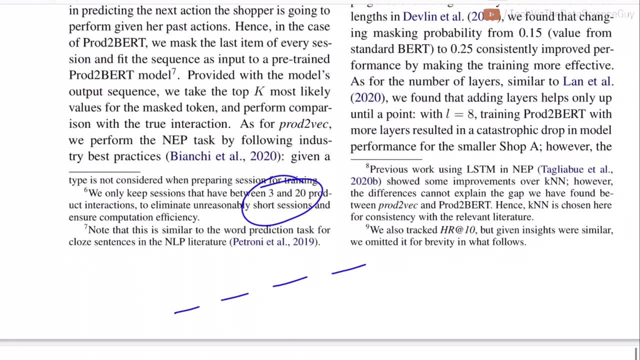 where the task is to predict the next action that the user is likely to take, given some previous actions. So it could be like if I come to the website, I just explore, explore then buy, then explore, then buy, or maybe one of the actions that's again over there. 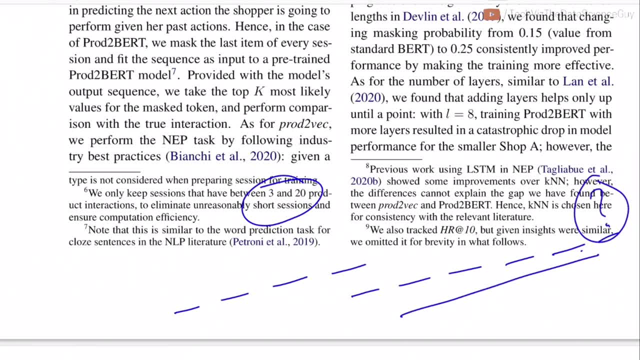 So what could be the next action that you predict? So this is like the next event prediction based on the previous events. what is the next action that I'm going to take? So for prod to BERT, which is again a BERT-based architecture, 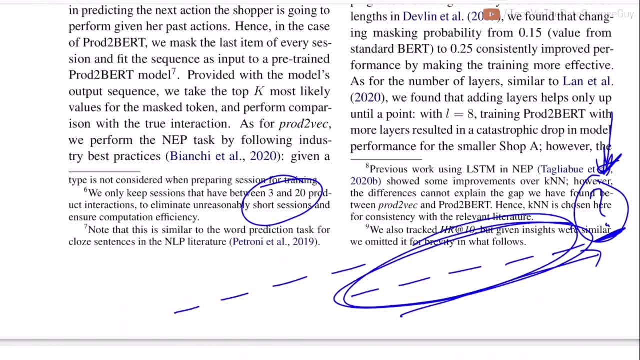 that we have discussed. they mask out the last element in every sequence and which is what the BERT is supposed to predict by seeing all the sequence tokens that have occurred in the past And at that T-th step we pick the top K, most likely action that the BERT says. 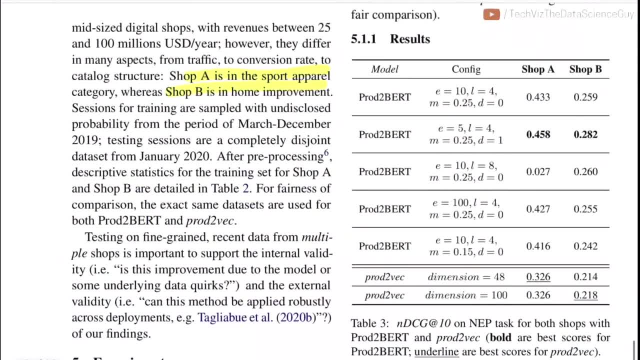 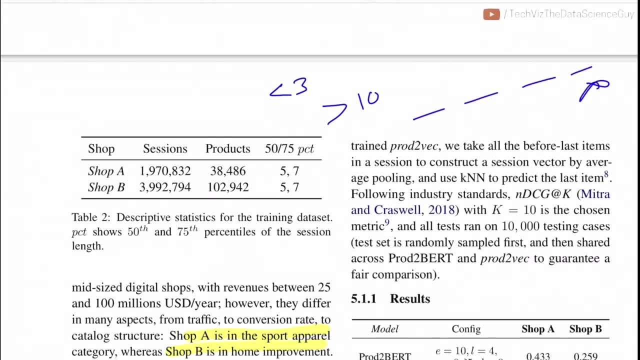 So that's about prod to BERT. Now, talking about prod to WIC, which is a word to WIC-based idea, we have a sequence of this sort, Leaving the last one, we take the representation of each of these actions, then average them out to get a one to T minus one. 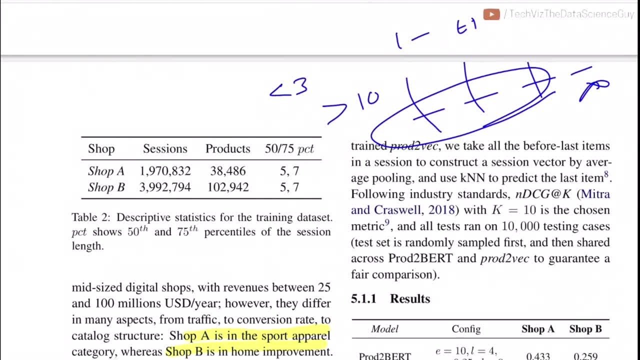 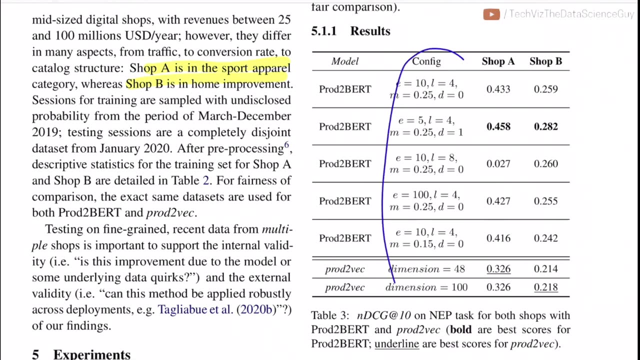 action, representation of our session, which they then use and perform the KNN prediction to get the last item, what is likely to be there, Share. these will include things that they tried and these are the results. with respect to that we can clearly see, based on different configuration. 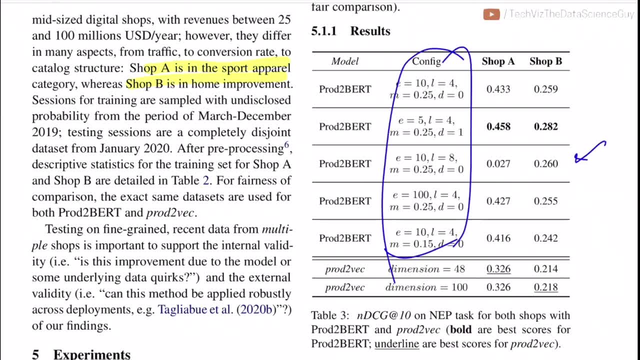 for prod to BERT. Almost all of them, apart from just this one, Surpass the best models for prod to WIC for both the shops by huge margins. We can clear this up with this, ok, And talking about the time it takes and the cost associated for trading, 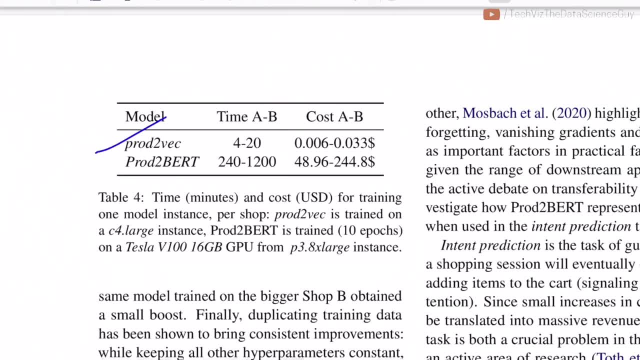 one of the model instances so far for prod to WIC, we can see the cost of purchasing A block value mobilitytt. So for Prod2Vec, the time it took was roughly around 4 to 20 minutes and the cost associated was $0.006 to $0.33, whereas- which is very high- in Prod2Bird to 1200 minutes and it costs 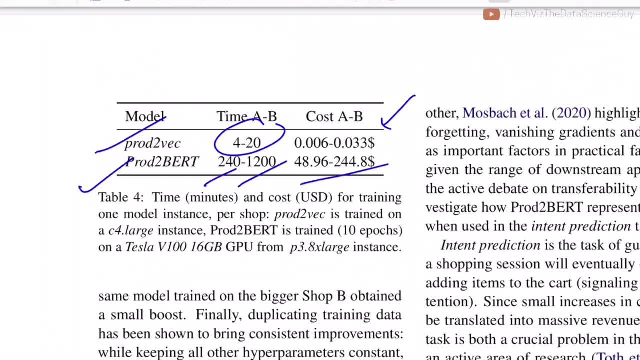 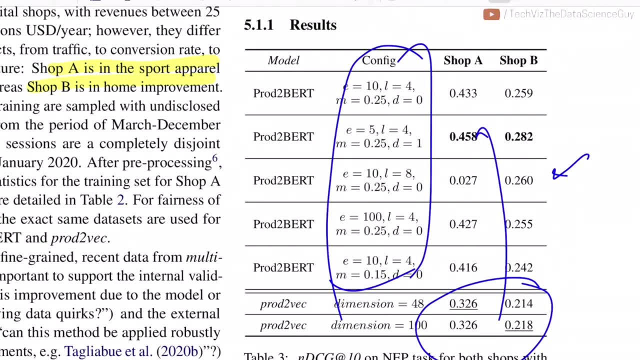 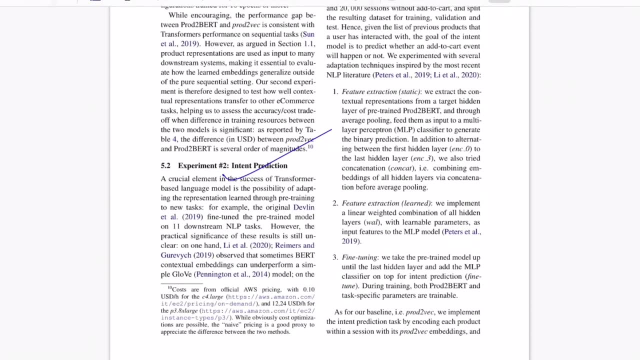 you somewhere close to $48 to $250.. So this is the trade-off that you get for getting the accuracy boost roughly around 10 point increase. So, apart from this, they did a second experiment, which is intent prediction, where the ultimate goal was to see if the shopping session is going to end in a purchase intent or not. 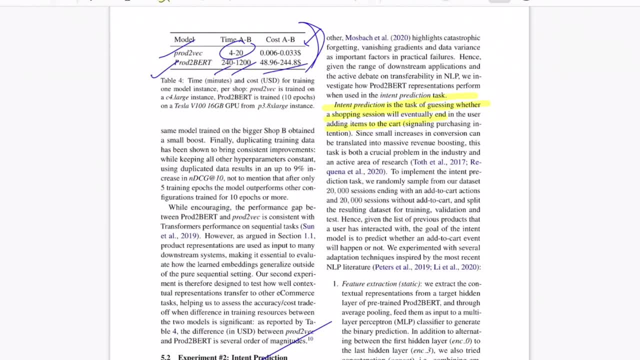 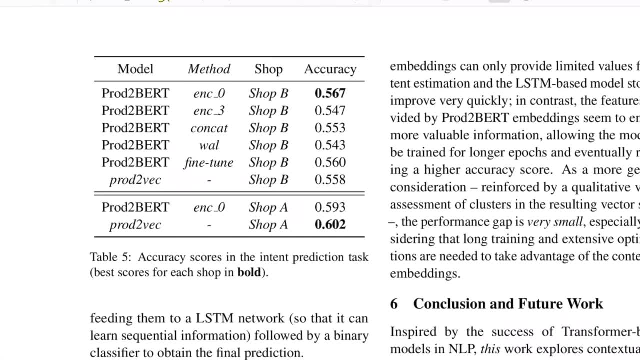 So that's what we had to classify, based on the representation that we learned for that session using Prod2Bird or Prod2Vec. So in this evaluation they found a little discrepancy in terms of the performance, which is all the next event prediction, as in various techniques, to how did they get the representation? 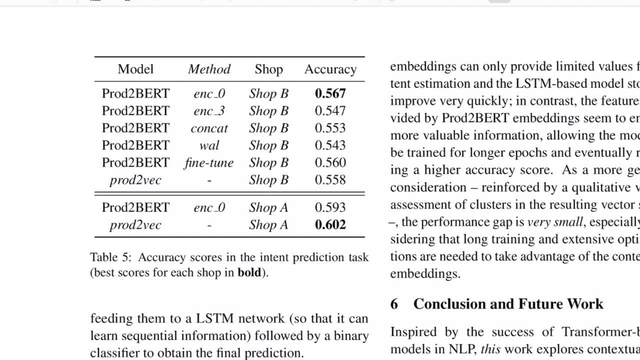 for the sequence. For example, one of the ways they picked in the representation was from the very early layer, from the bird. Then the second was to concatenate embeddings that you get from every layer, then learning a function that would merge the embeddings from the last layer into one single representation. 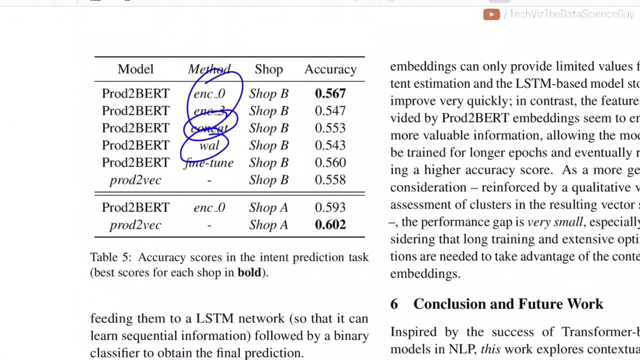 and finally, adding an extra layer on top of the CLS vector and then fine-tuning the entire architecture. So all of these were the experiments that the authors tried in terms of evaluating the goodness of the representations. But still, if you see the accuracy numbers, Prod2Vec gave us 0.558, and the best one from 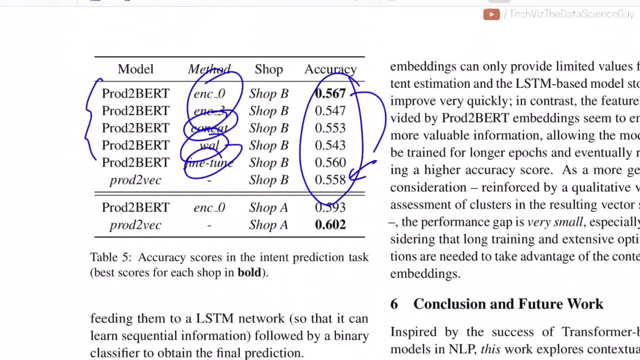 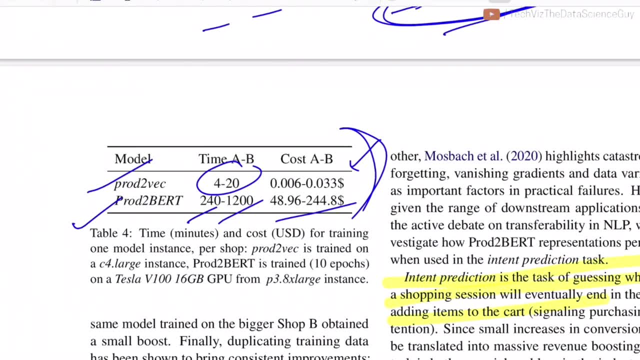 Prod2Bird gave us 0.567, which is almost a negligible difference. But if you see the trade-off in terms of time and cost it takes to train Prod2Bird compared to Prod2Vec, clearly Prod2Vec is the choice that you want to make right. 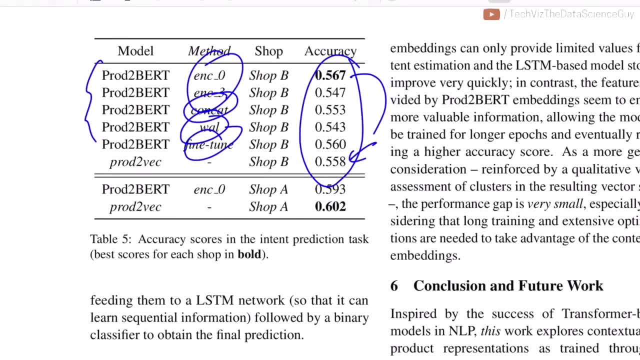 So, yeah, that's the trade-off and clearly I feel it's not really a confident conclusion in terms of knowledge. However, based on these guys' discussions with Prod2Bird and Prod2Vec, I simply believe that Prod2Bird and Prod2Vec will, show-short- perform better for a given task. 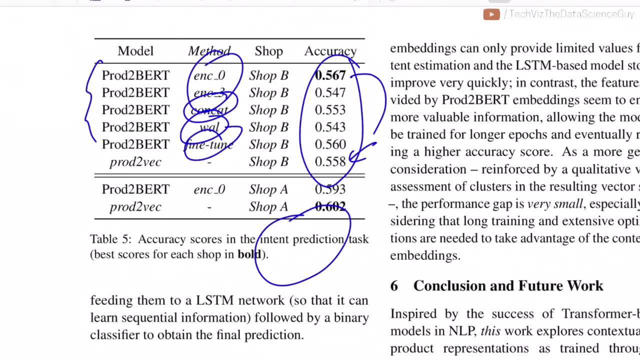 Because that's what we are seeing in an intent prediction task and the next event prediction. One of the hypotheses that the researchers make in this paper is that probably the Prod2Bird performs really good in any retask because the behaviour of the task is more or less. 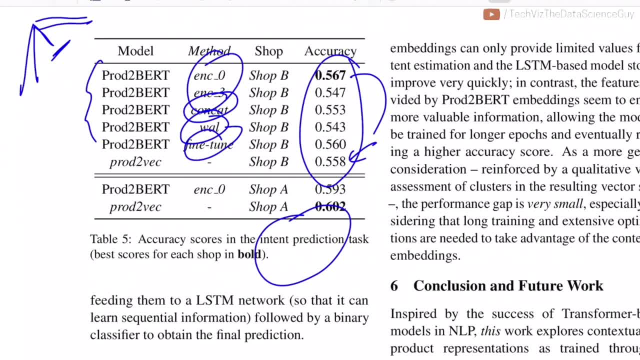 like MLM, where you mask out something and predict that based on other things that occur to its context mask, you consider bidirectional context for making this prediction and in the next even prediction tasks, you specifically just mask out the last token and make prediction based on the tokens. 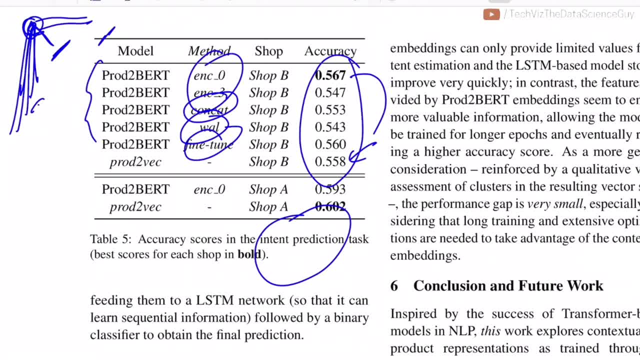 that are towards left. but still the idea is same, because in the original mlm training the model would have seen such scenarios as well. so that's why fraud2bird performs better than fraud2vec for that specific task, which is unlike the case in intent prediction, because this is just a. 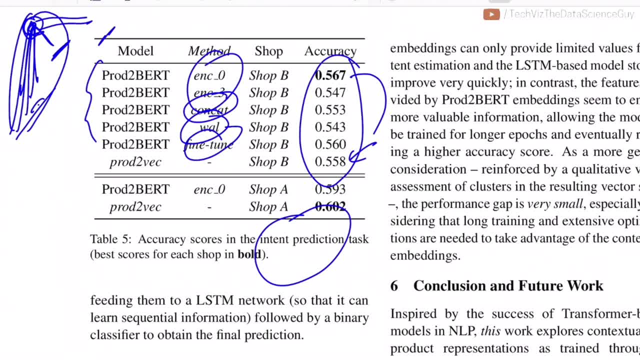 sequence classification task. but probably, i believe, if nsp was also tuned, which is next sequence prediction, apart from just the mlm, then we would have seen gain in the internet prediction task as well, at least for fraud2bird fine-tuned segment. so yeah, i think now we are done with the